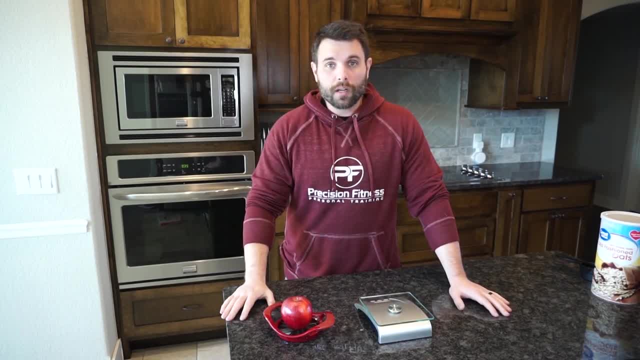 need. What I'm going to do is I'm actually going to link below in the description to one on Amazon that you can pick up. They're only about $10, but you can really get them anywhere. You can pick them up at Walmart local store. I'm going to show you how to do that. I'm going to show you. 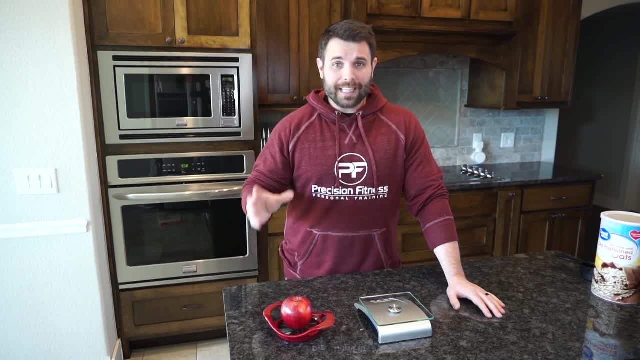 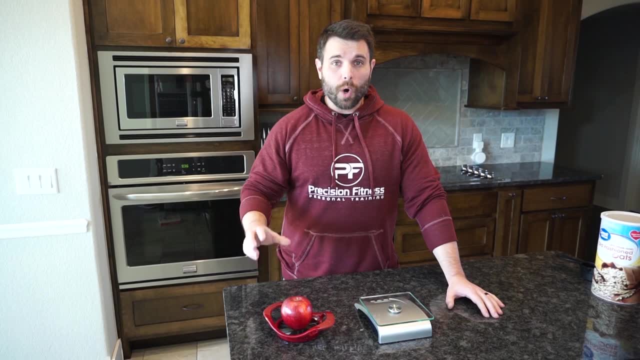 or use the link below to pick one. $10 is a pretty good one. They last forever and I have had mine for years and I've never even changed the battery out of them. Pretty easy to use. The first thing that I want to do is actually go over the scale and explain how it works, just in the basics of it. 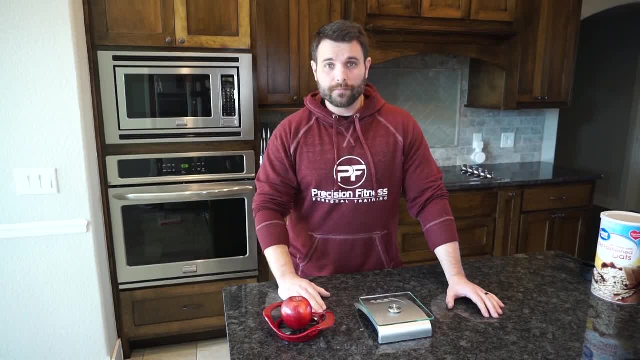 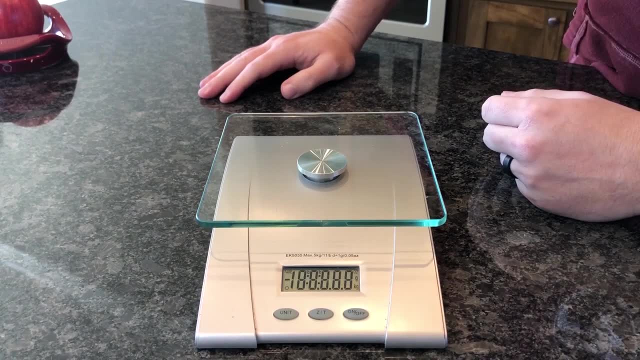 and go over the few buttons so that you understand all of the basics of using the scale. Most of these scales are going to have anywhere between two and three buttons. Of course, you've got your on-off switch to turn it on. Then you're going to have your ZT, which essentially means to clear it. 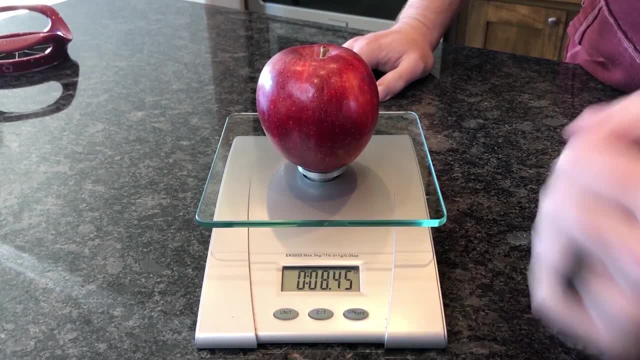 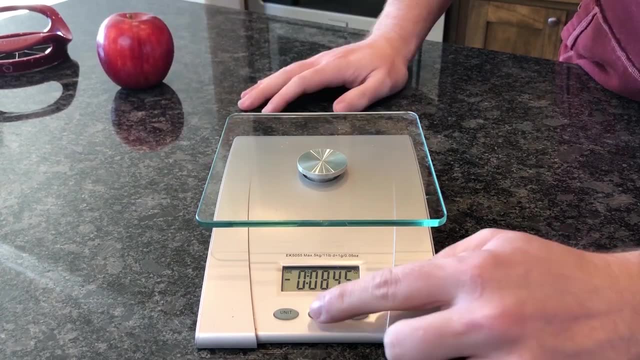 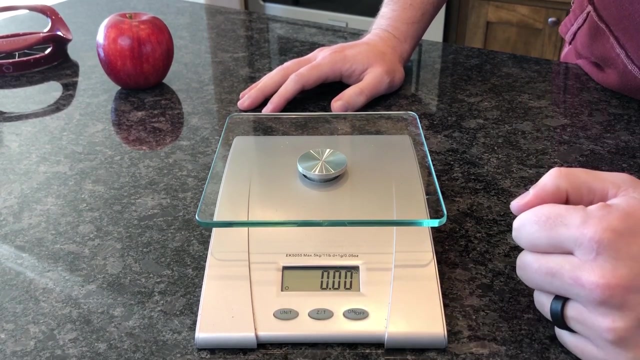 If you want to clear it out, you can click this and it goes automatically back to zero weight. Same thing: take this off If I wanted to clear it back to zero. that takes that. The other thing is the units. Right now it's set up in pounds and ounces. From there you've got ounces and from 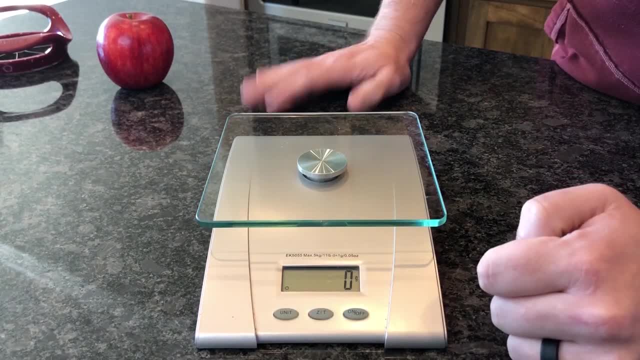 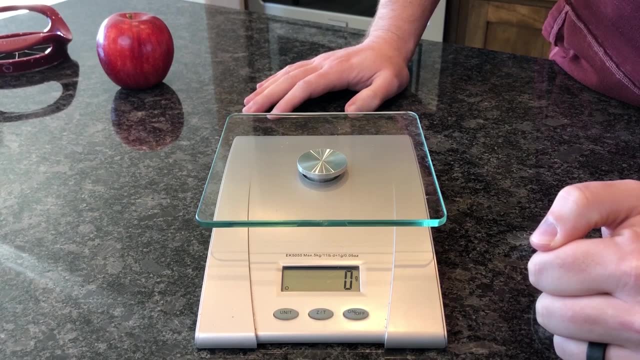 there, you've got grams. Now, whenever doing any type of weight measurement, I highly recommend that you really only use the ounces and the grams feature. These are the only two that I recommend whenever you're going to use the ounces and the grams feature. These are the only two that I 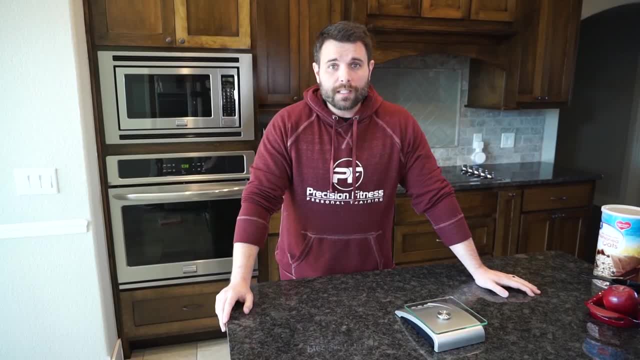 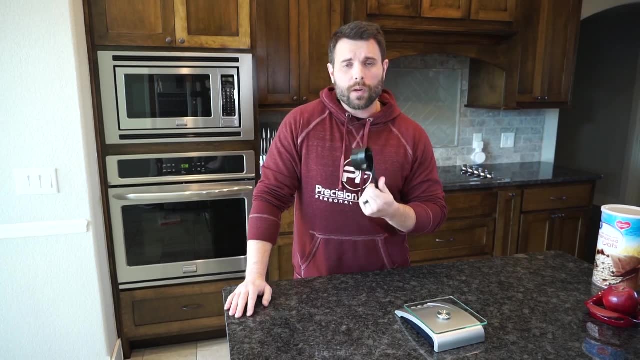 recommend when you're trying to weigh your food and use these scales. Now, the reason that I said that I only recommend that you use scales and not measuring cups is because whenever we are weighing and measuring food in order to be accurate, it's really important that we are weighing by weight. 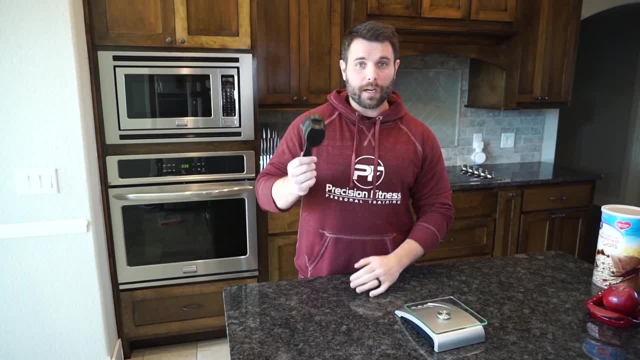 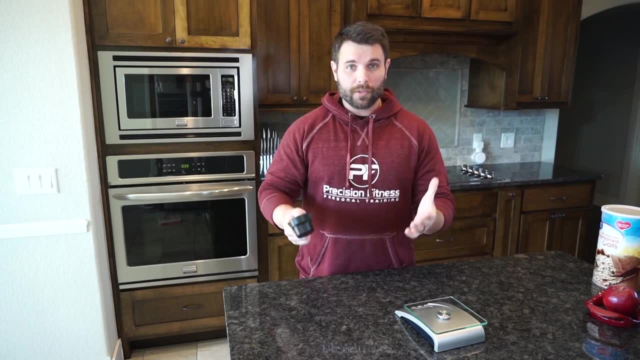 and not by volume, as this can be an inaccurate method. Whenever you are just a little bit inaccurate multiple times a day, it tends to add up Again. going back to if you want to do this accurately, if you're going to take the time to do it, you want to make sure that you're doing it. 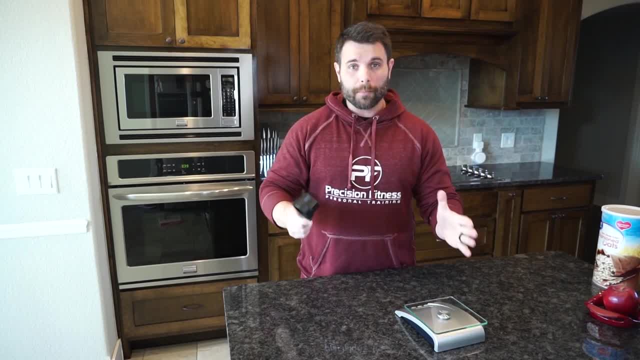 right. I typically don't use the ounces and the grams feature. I'm going to use the ounces and the grams feature. I usually use the scale. I'm going to give you an example and show you why that's the case. The example that I'm going to use here and explain to you why I always use the scale instead. 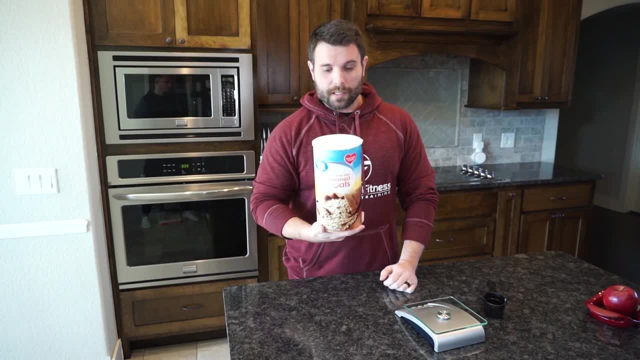 of measuring cups is. I've got some oats here. I'm going to use this as an example. If we look at the back- and I'll show you this here in just a second- it says that a serving size is half a cup dry. 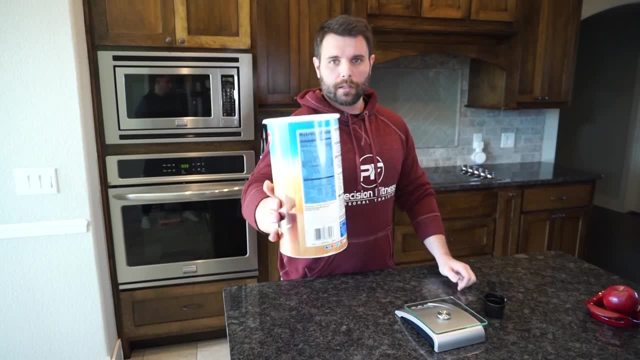 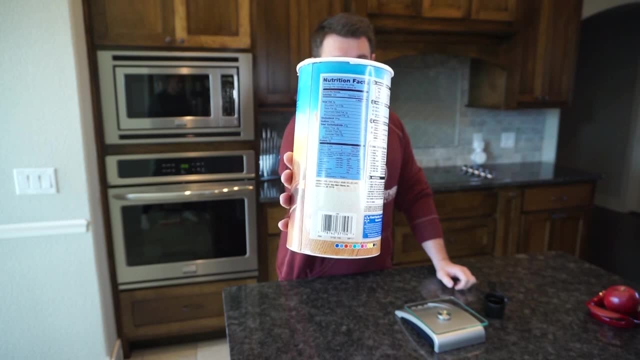 which is also 40 grams in weight. If you take a look at this and you can see it's about half a cup for a serving size, and 40 grams in weight is what we're looking at here. If that was the case, what I'm going to do is sit this here on the scale. 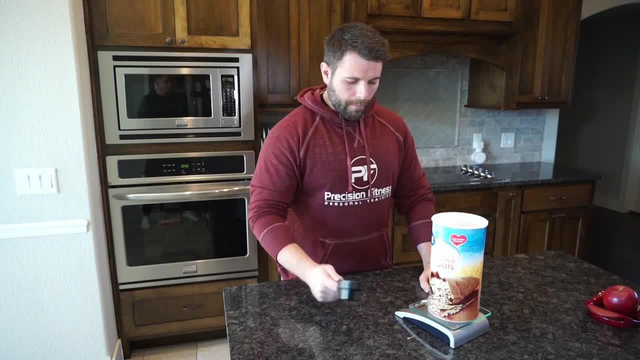 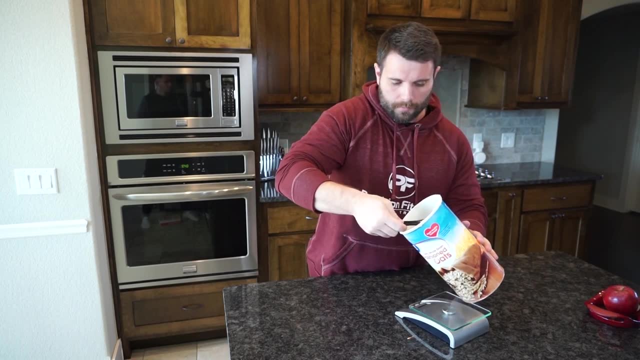 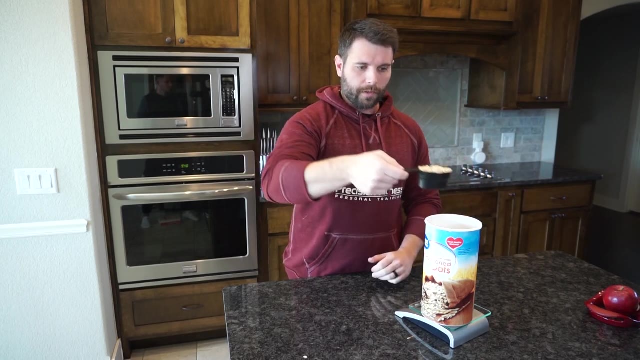 and turn the scale on so it's automatically zeroed out. I'm going to hit the unit button a couple of times to make it go over to grams. I'm going to take out what would be considered about a half a cup. That's a pretty level half cup. It's not overflowing by any means. 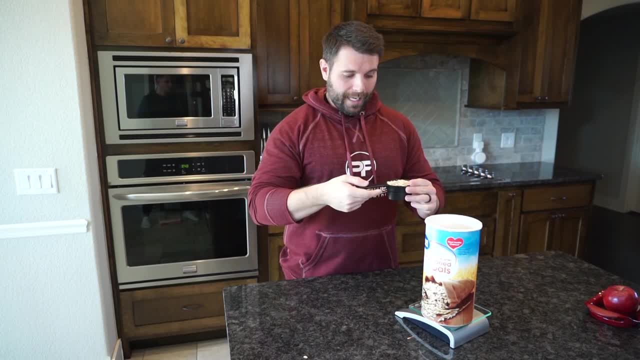 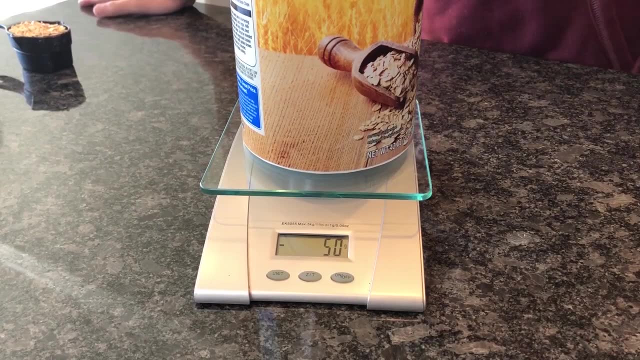 pretty good half cup. If you actually look at the scale, it's saying that this is 50 grams in weight. You can see here that it's 50 grams in weight, even though it says that a half cup is only supposed to be 40 grams in weight. 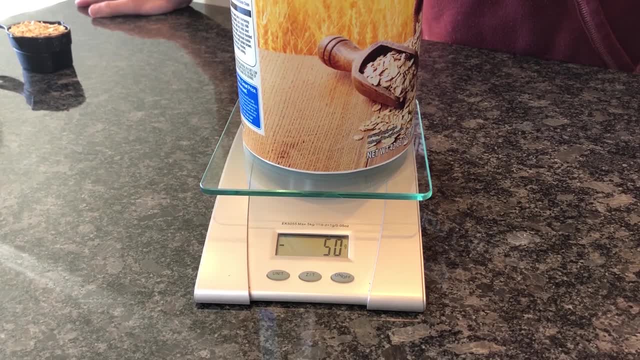 That's a pretty decent increase in calories if you were just doing one serving size. If you did this for two serving sizes or three, it would continue to get worse the more of this you ate. This is why it's really important that we are weighing by the actual weight and not by the 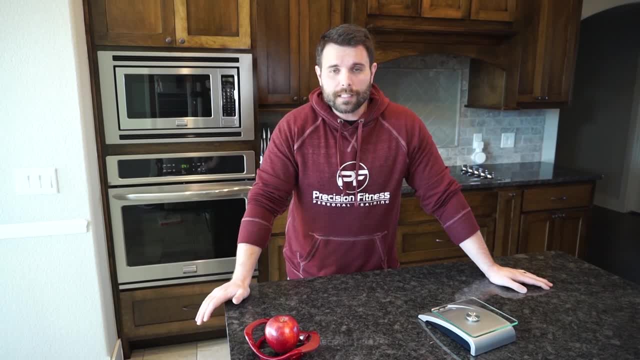 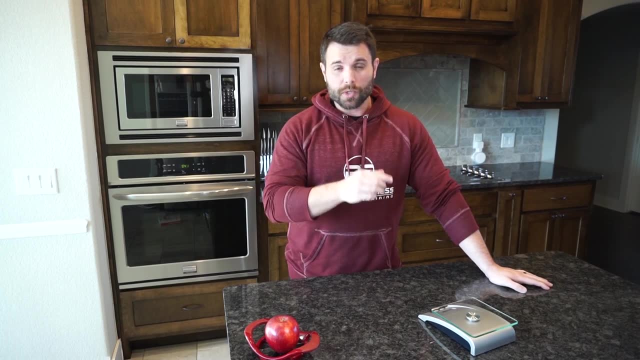 volume. Another thing that you want to pay attention to- and it seems almost silly to mention this, but it's also really easy to overlook this- That's that you want to make sure that, when you are weighing and measuring, that you're only measuring what you're eating. Let me give you 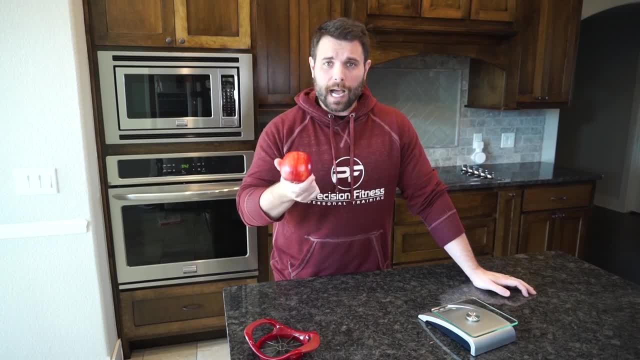 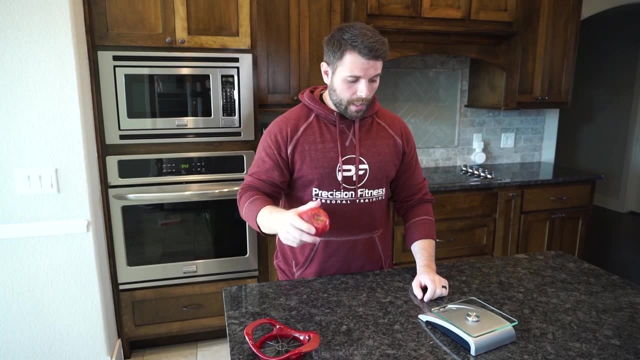 an example here. Let's talk about this apple. If somebody was to eat an apple- it's not uncommon- Somebody might weigh the apple to see and get an idea of how much it weighs. They turn the scale on. They turn it to either ounces or grams. I'm going to go ahead and put grams When I sit this. 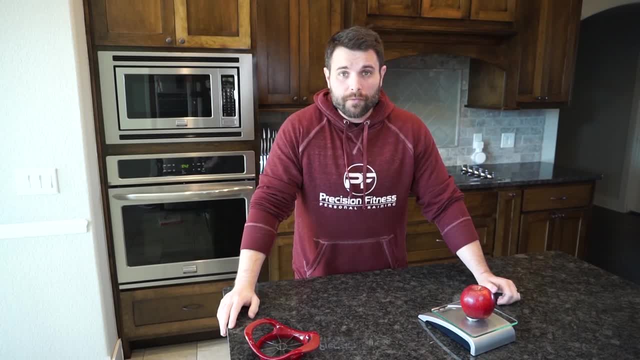 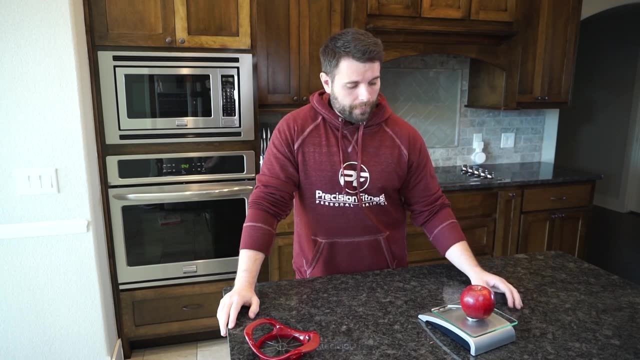 on the scale, it currently shows that this apple weighs 240 grams. If you were to put that in there, you would weigh 240 grams worth of apple. if you put that in your tracker Now, the downside of that is I'm not going to eat the whole core. I'm not going to eat this. It's going to make. 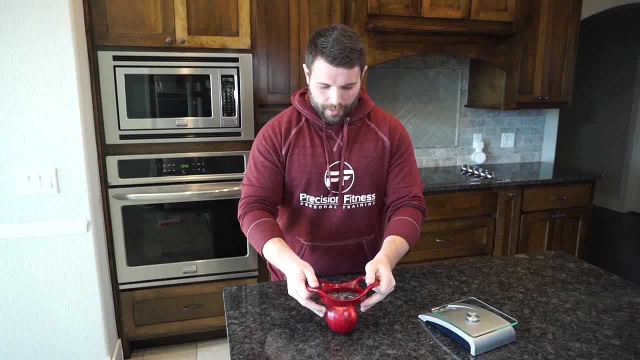 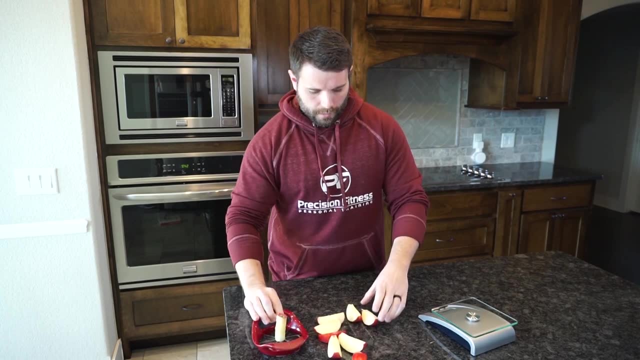 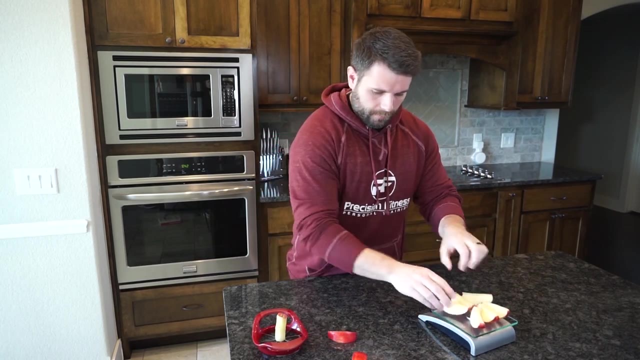 a difference If I use my fancy little apple core slicer here. cut this, knock these off. Typically, I would have a plate here. I just don't happen to have one on me at the moment- but sit the pieces of apple here on top of it, because this is what I'm actually going to eat. 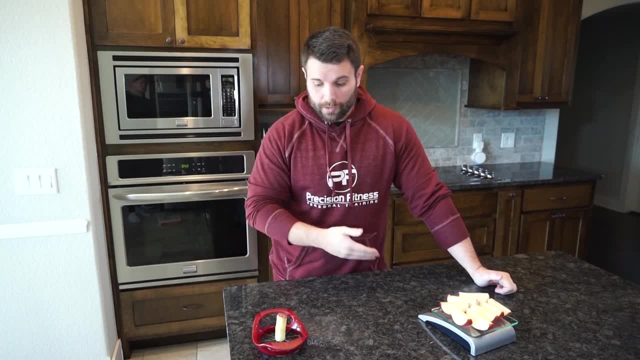 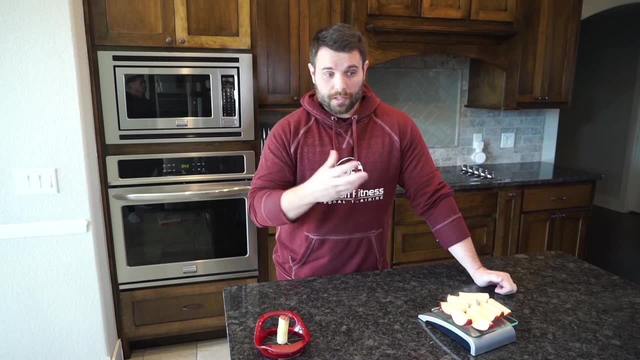 We've now went from 240 grams down to 214 grams, because the core that's left over in here I'm not going to be eating. This is the part that you want to measure. This is going to go with pretty much anything else that you put in there. Think about a banana. You don't want to weigh the. 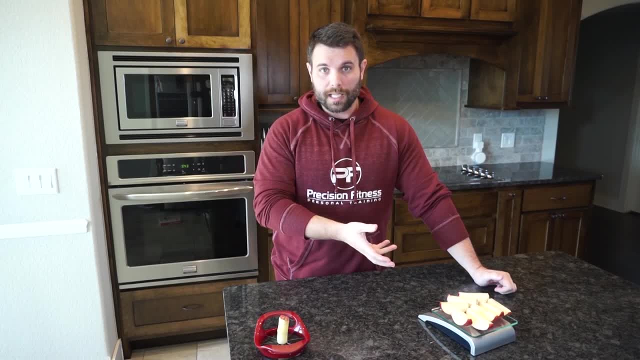 whole banana. You're going to take the peel off and you're going to measure just the part of the banana that you're going to eat. Make sure that that's something that you're considering whenever you're weighing your food. Another thing to consider is whenever it comes to weighing and 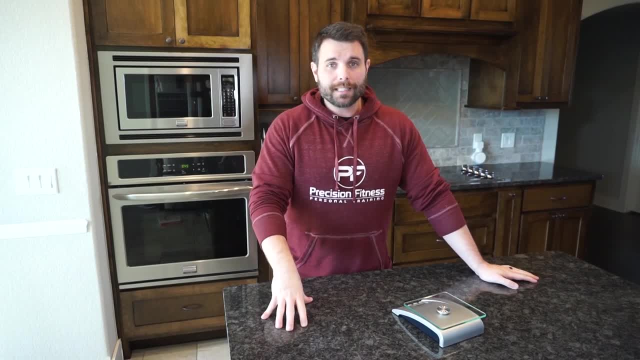 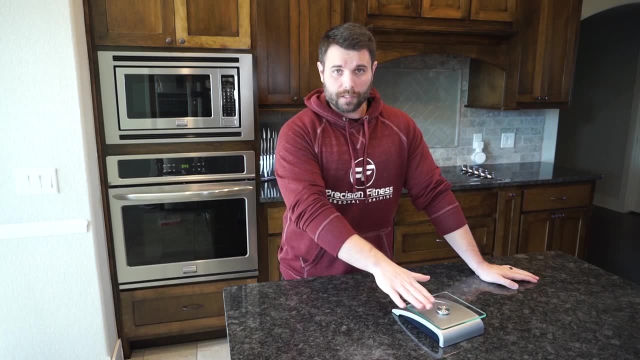 measuring your liquids. Now here's the thing that I highly recommend is that you do this based on the weight. Whenever you put something on the scale and you move the scale over to ounces, it's measuring it in ounces by weight. Now, if you look at, whatever you're drinking, 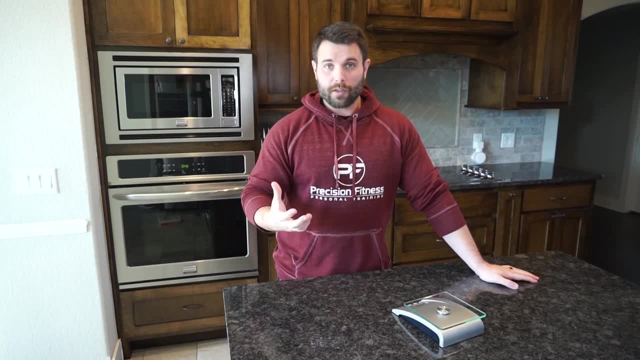 if it's milk or orange juice or whatever liquid you're potentially putting in there that contains calories that you're trying to measure. most of the time, it's telling you the serving size based on a fluid ounce. A fluid ounce is based on the volume of what you're drinking. 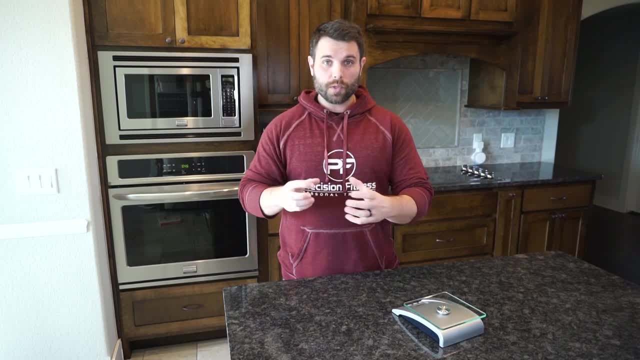 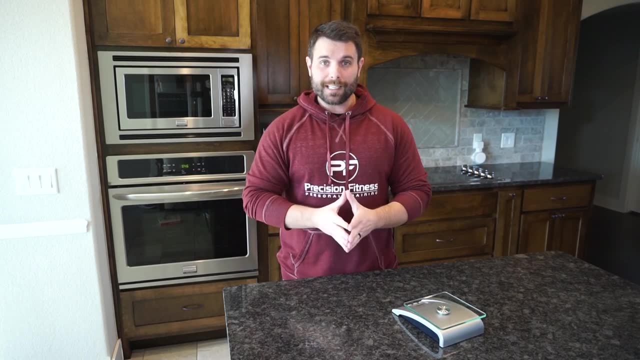 12 fluid ounces of orange juice is not going to be the same as 12 ounces in weight of orange juice. It's going to be different. So anytime that you are drinking something, any type of liquid, that contains calories, I highly recommend that you weigh it by grams. 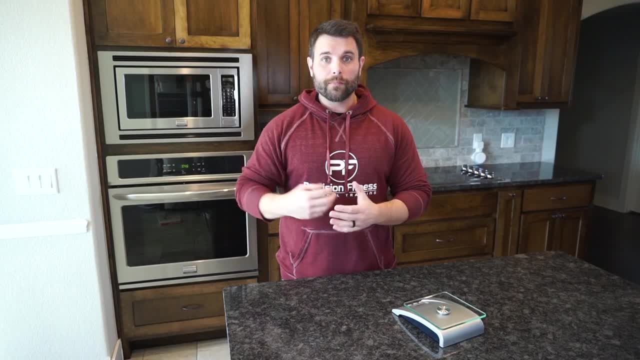 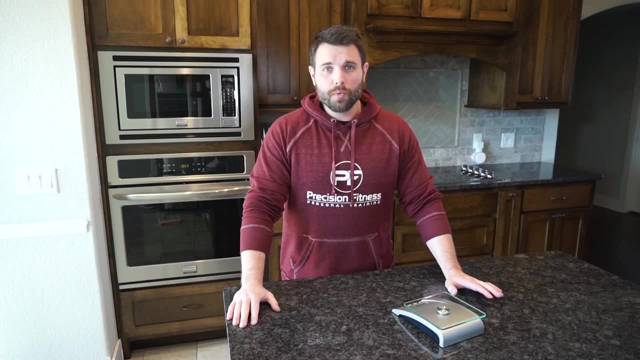 in order to be accurate And then when you put it into your tracker that you are putting that in there as grams so that you know that you're doing it a hundred percent on point. Another question that I get asked a lot is: should you measure your food raw or after you cook it? 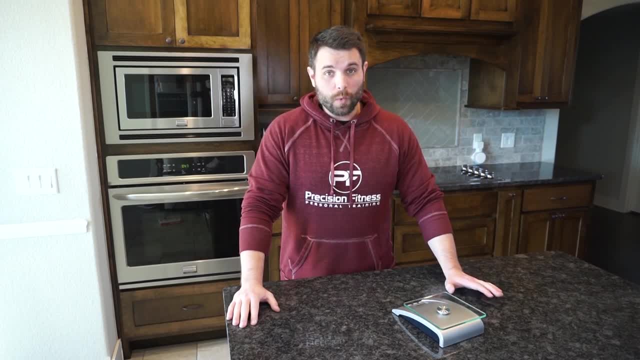 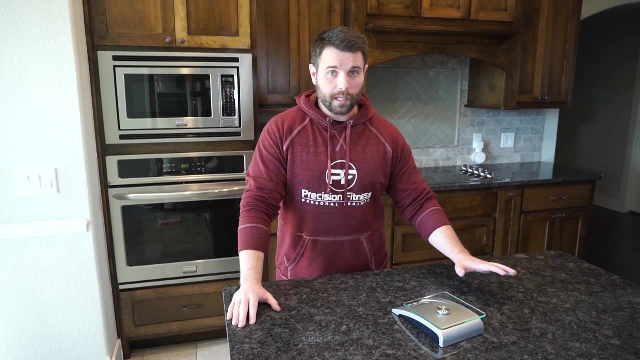 Now here's the thing. Either way is fine and either way can work. My first recommendation is to be consistent with it. Don't go back and forth in doing it raw and measuring it one time and cooked another time. Make sure that you are being consistent in the way that you choose to measure. 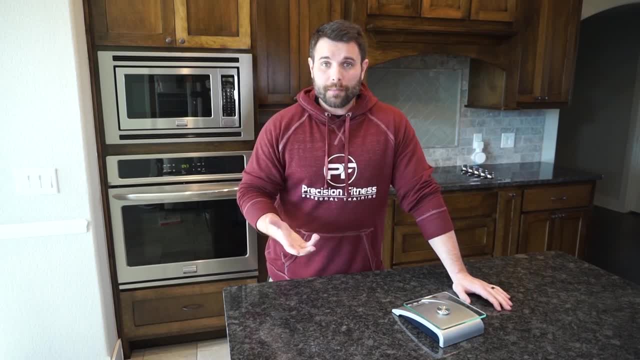 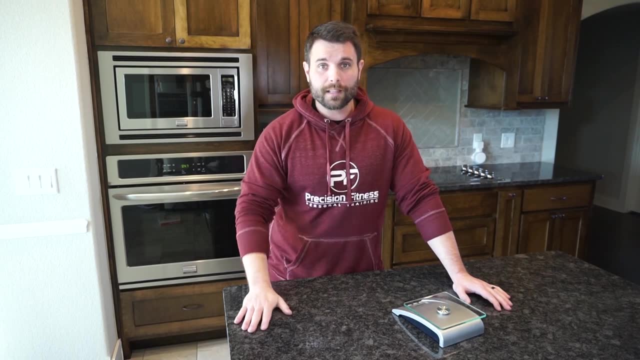 it either way. From there my personal recommendation, not a requirement. what I have found easiest for me, and typically for most of my clients, is to measure it raw. So a couple other things to think about here. If you were cooking chicken or beef or something like that that you 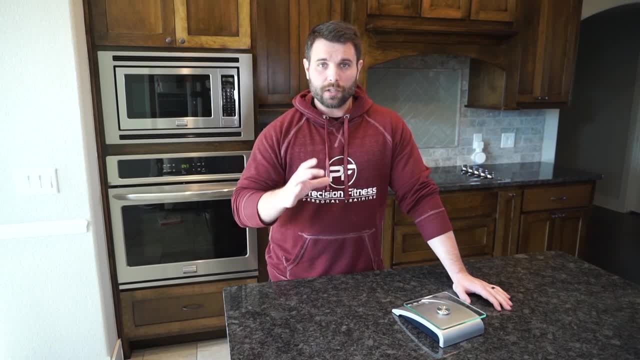 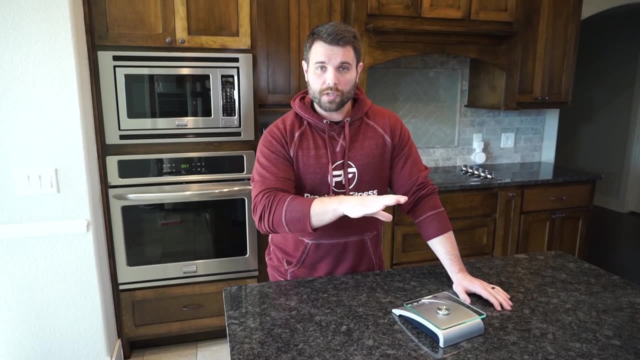 know that you're going to have to cook when you look at the information on the back, the nutritional information. So if you're using your app to scan it and you're trying to be accurate with that, it's giving you the nutritional information based on it being raw. So the easiest way is if you are cooking five or six ounces of. 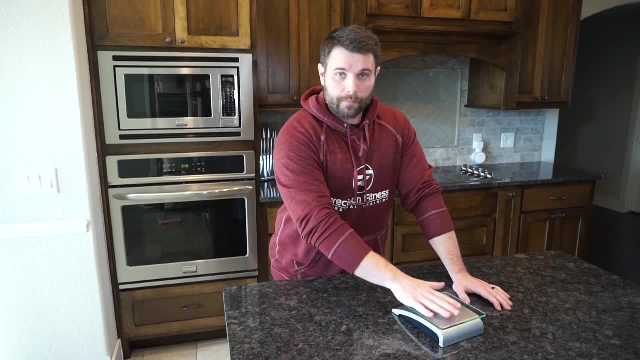 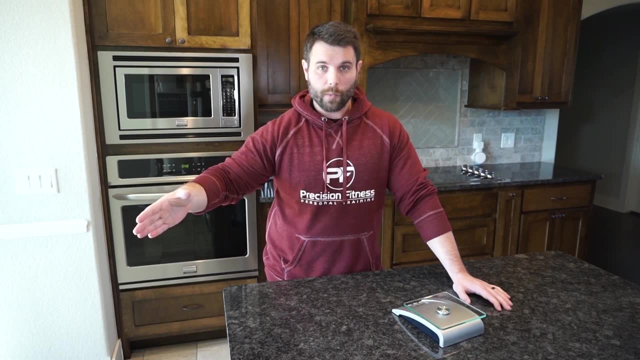 chicken is to weigh out five or six ounces of chicken on the scale and then input that into your tracker as five to six ounces of chicken, and whatever it comes out to be, it's still the same. You don't have to worry about re-weighing it The only time that this is going to be an issue that. 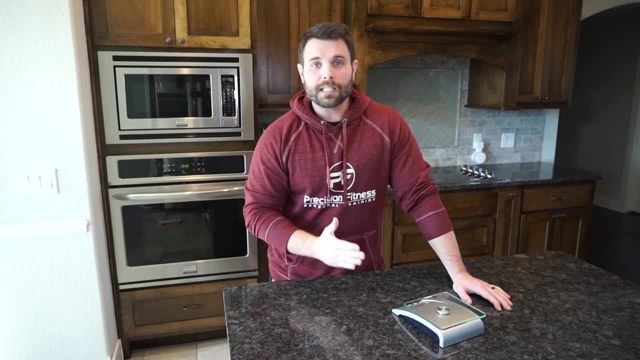 you have to do just a little bit of math. not very much, just a little bit- is if you are someone that cooks in bulk, If you are someone that cooks in bulk. if you are someone that cooks in bulk, so if you, on Sunday, you decide to cook all your chicken for the entire week and you have to 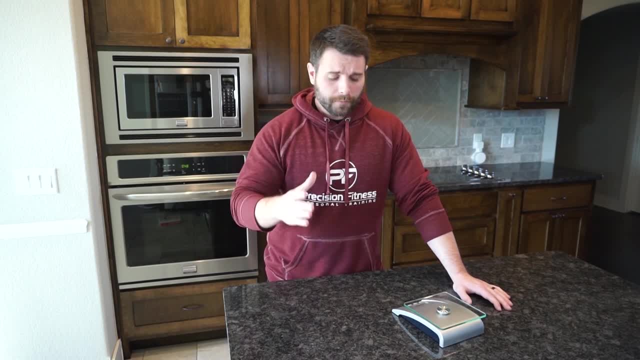 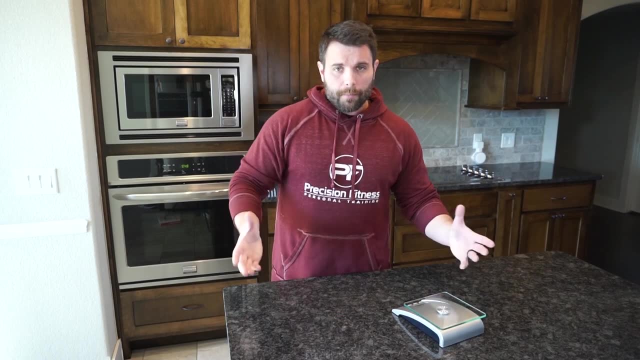 portion it out from there. this is where you're gonna have to do a little bit of math. So let me give you a little bit of example. So let's say that you're cooking some ground beef and you're making it for the week, And whenever you lay all the ground beef out that you're going to cook, 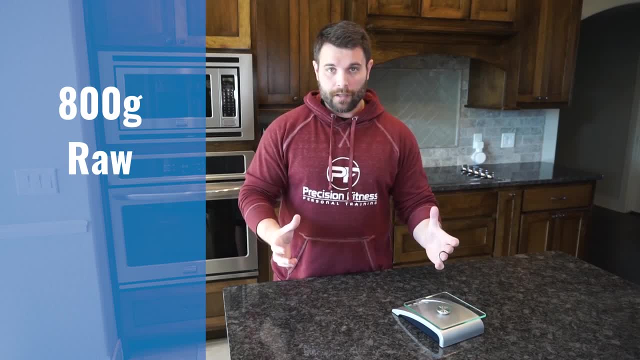 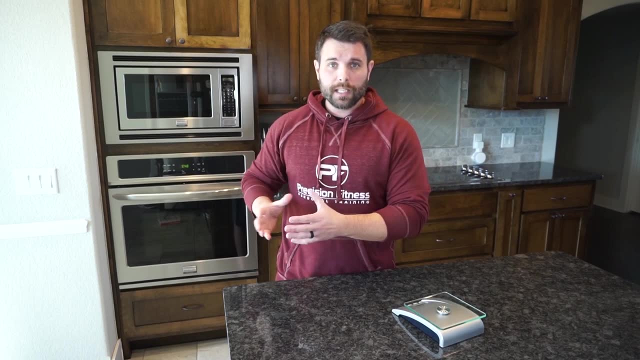 it is 800 grams worth of beef. All right, So what you would do is you would take that number, that 800 grams of beef, and you would write it down after you cook it. So once you've cooked it and you've drained it and what you have left, 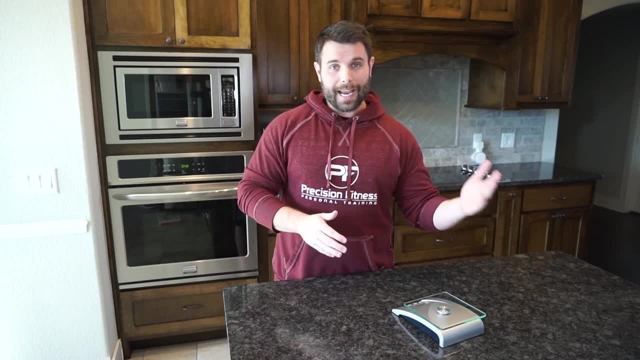 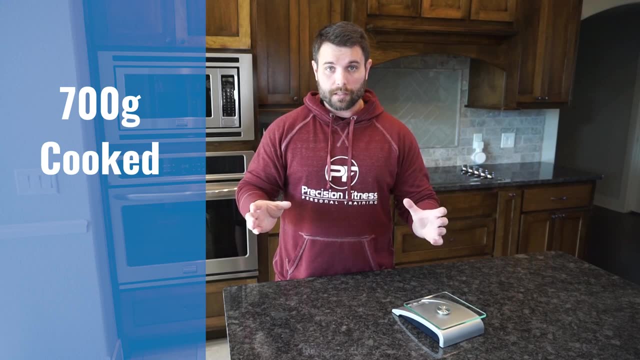 you're going to weigh it again Now. I'm just making up numbers here. but if you had 800 raw after you cooked it, it dropped to 700 grams raw. So you lost a hundred grams in weight. based on doing this, What you're going to do is you're going to take 800 and divide it by 700. 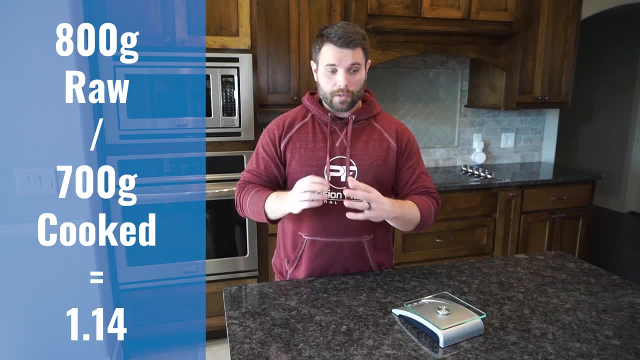 When you do that, you're going to get 1.14.. So you're just going to have to remember that 1.14, and then you will put your meals in the fridge, do whatever you're going to do with them: freeze. 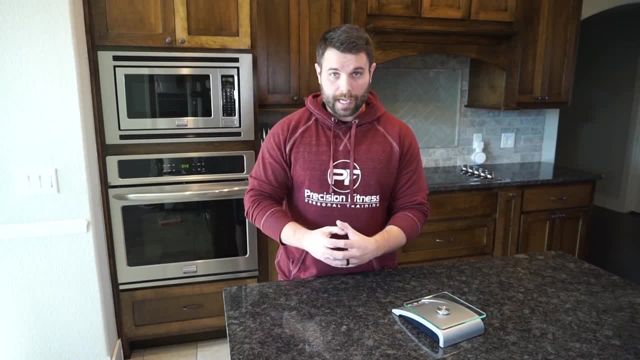 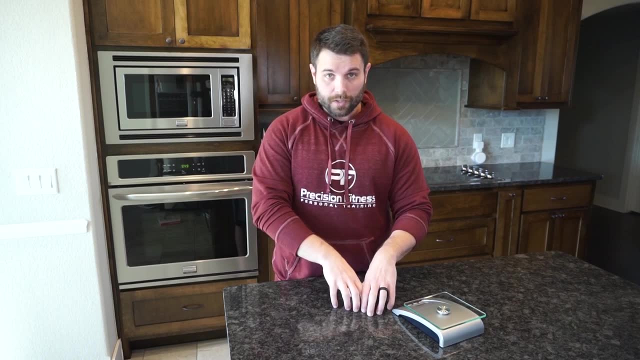 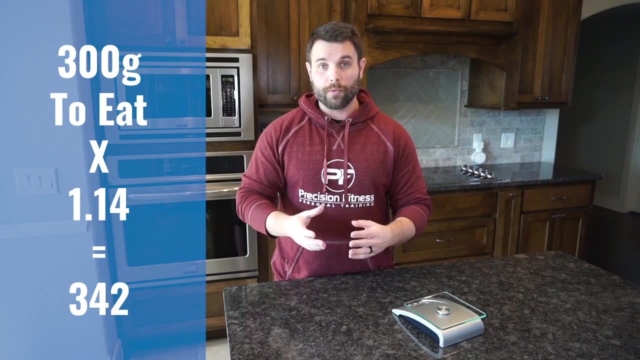 them When you pull the meals back out, however much you take out. So let's say that you decided to take out 300 grams worth of that, 700 grams is left. You would take that 300, the amount you took out and multiply it by the 1.14.. Whenever you multiply that by 1.14, you're going to get 342.. 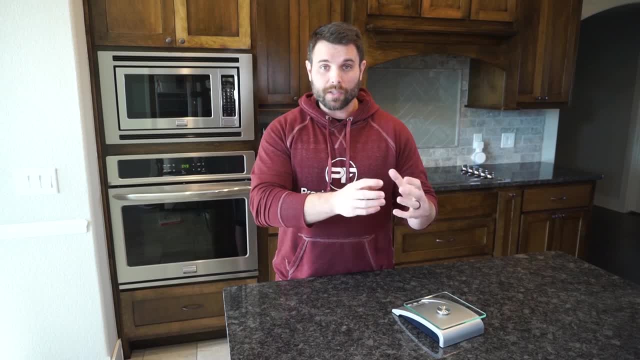 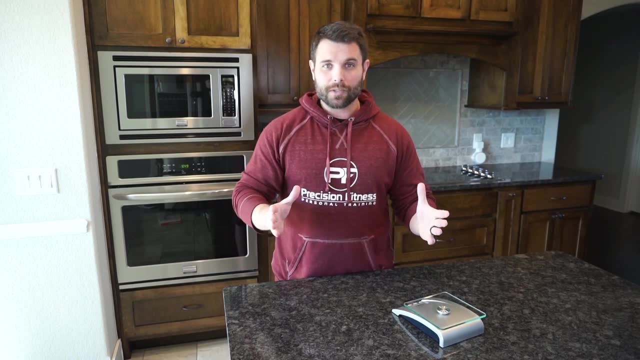 So that would be the number that you would enter into your tracker, based on the raw weight. Hopefully that makes sense. It'll make more sense if you actually go through the process. it's not complicated. It'll take you like an extra minute or two to do the math.